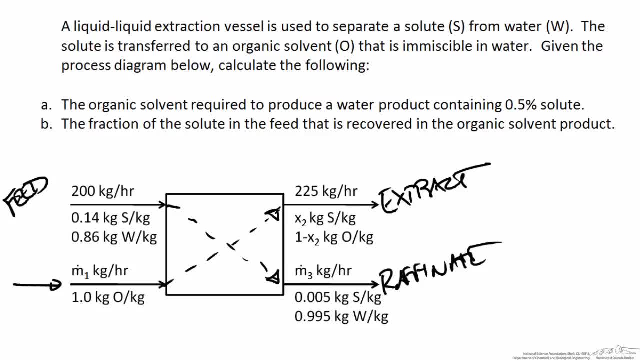 The solvent that's been enriched in the solute is known as the extract. Given our process diagram, we're asked to calculate two things. Number one: we want to find the organic solvent that's required to produce a water product containing 0.5%. 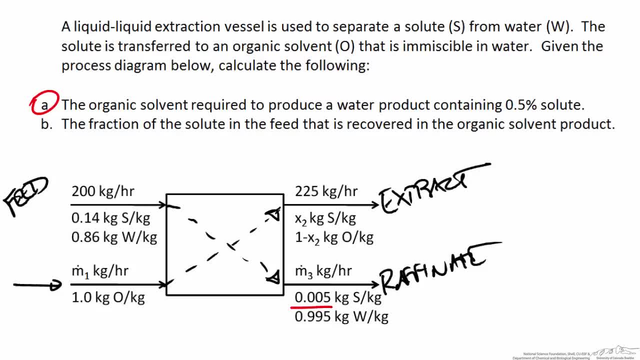 solute. So that's indicated by the mass fraction of 0.005S in the raffinate and we want to find M1.. The second thing we're asked to calculate: we want to find the fraction of the solute. 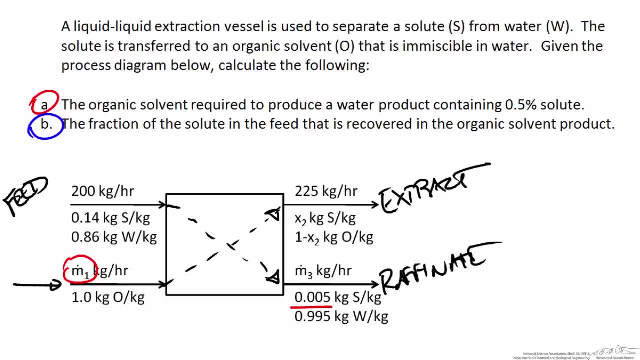 the feed that's recovered in the organic solvent product, which is the extract. so of the solute coming in, how much of it ends up in the extract stream? so to do that, we're going to have to find a value for x2 before we start setting up a system of mass balances and calculating what 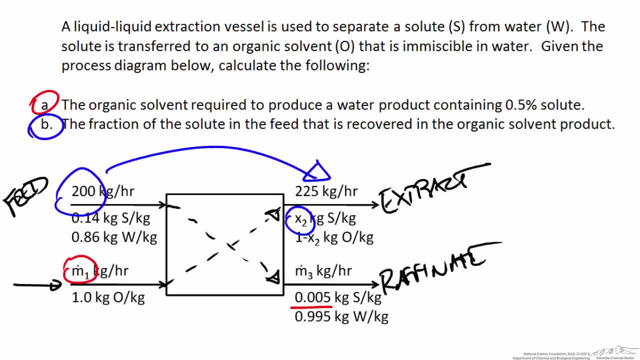 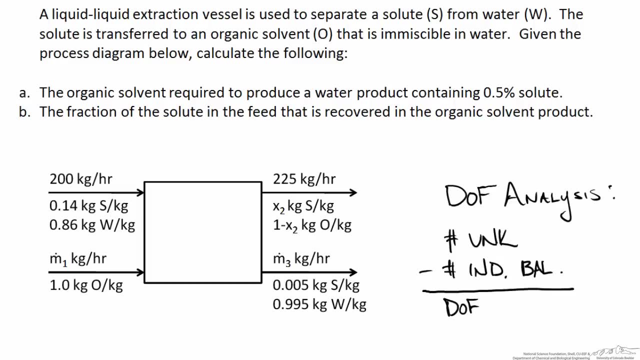 we need. it's generally a good idea to find out if we have enough information in the problem statement to solve for what's asked for. we can quickly determine whether we have enough information by conducting a degree of freedom analysis. the degrees of freedom for a process is given by the number of unknowns minus the number of independent balances that relate. 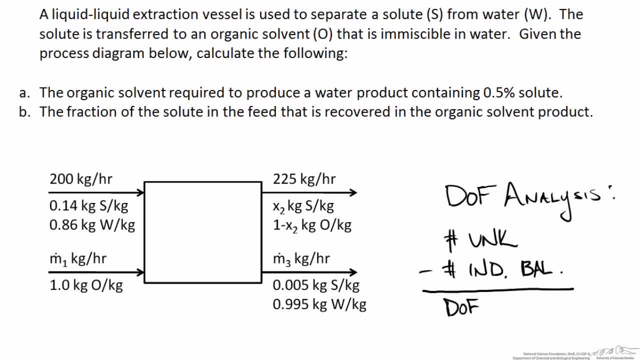 those unknowns. if we look at the process diagram, we can see that we have one unknown in m1, another in the composition, in the extract of x2 as well as m3. so we have three unknowns for this particular process and we know that we can write an independent balance for as many species as 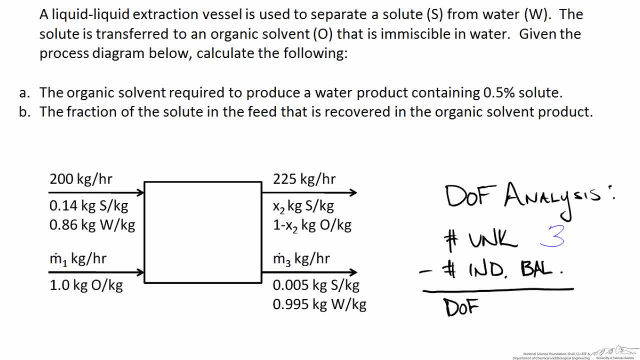 we have in the process. in this case we have three separate species, we have s, we have o and we have water. with three species, we can write three independent balances. technically we can write a fourth on the overall mass balance as well, but the total mass balance on the system is not independent from the species balance as it can be derived from summering up. 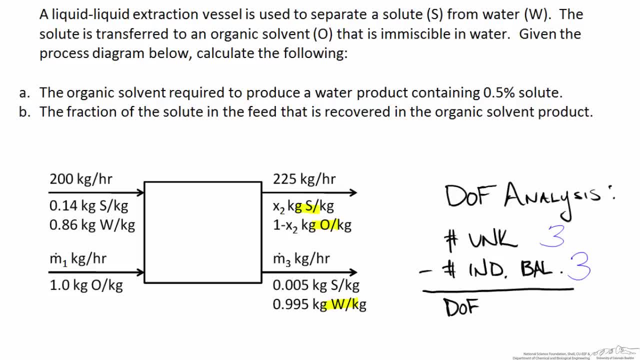 the species balance for every species in the system. so with three unknowns, three independent balances, we are left with zero degrees of freedom. in principle, we have enough information to solve for all three of the variables on this process chart to calculate the two things that are asked for in this problem. we 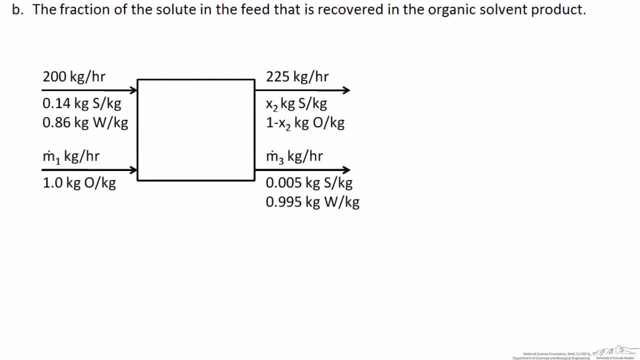 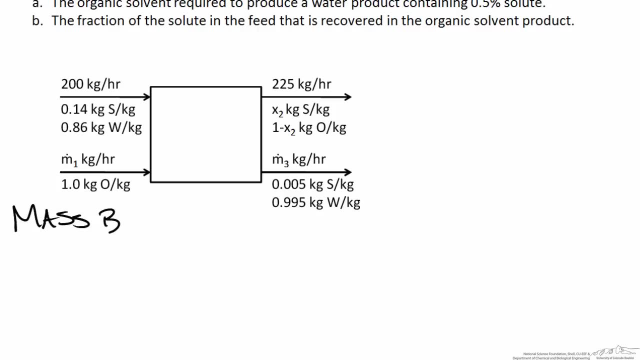 can relate the process variables with material balances. so the principle of the mass balance is conservation of mass, which is what goes in must come out. so all of our mass balances should have the form of n equals out, and we can write one on the total mass balance as well as the three. 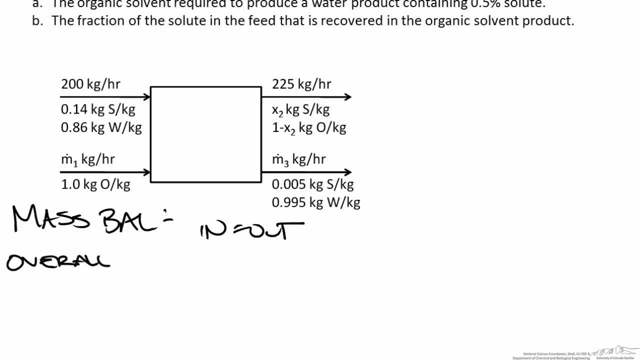 components in our system, for example, the overall mass balance. in this case we have 200 kilograms per hour in the feed, plus our unknown of M1, and that must be equal to what's leaving, which is 225 in the extract plus m3 in the raffinate. looking at the overall balance, we have an 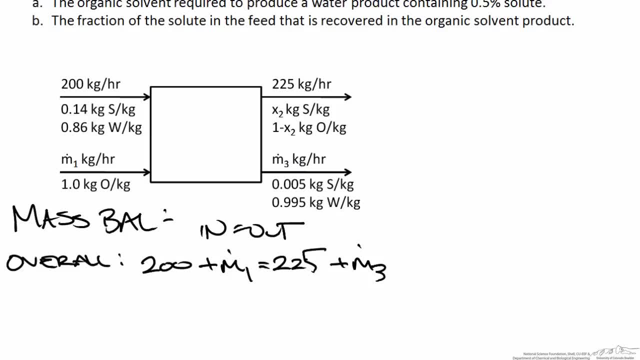 equation with two unknowns. so we're going to need at least one species balance to calculate you what we're asked for, which is m1.. So because we're trying to calculate the flow rate of the organic solvent in, we can use the species balance on the organic solvent which is we have pure. 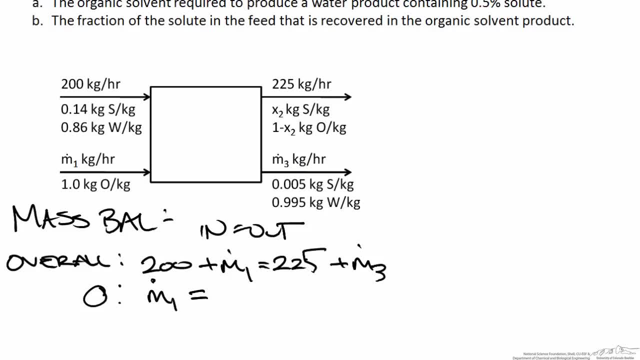 organic solvent in that stream. so we have: m1 is equal to 1 minus x2 times the total flow rate in the extract, which is 225.. Looking at the balance on the organic solvent, we can see we've introduced another variable, x2. so we'll need one of the other two balances, either s or w, Doesn't matter. 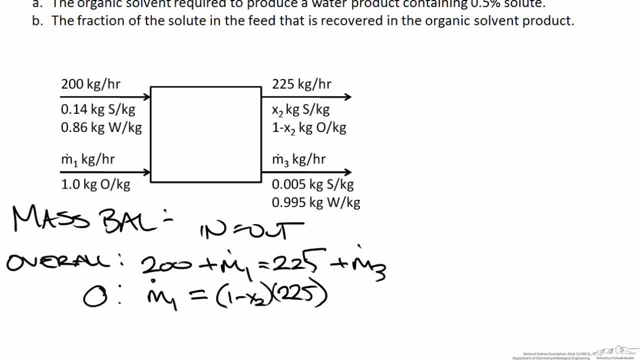 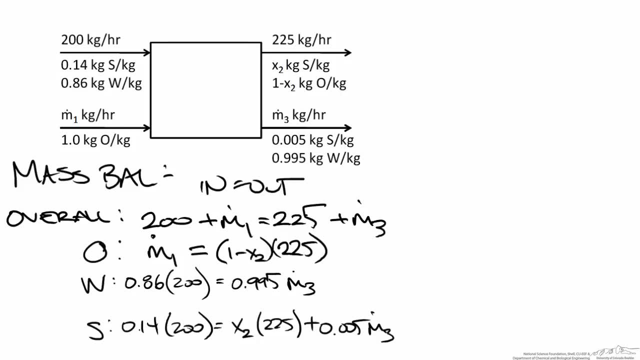 which I will quickly write both of those balances so we can see what balances is easiest to use to calculate what we're looking for. With both the water balance and the solute balance written as well, we can quickly look at the system of equations and determine which balances we can use to 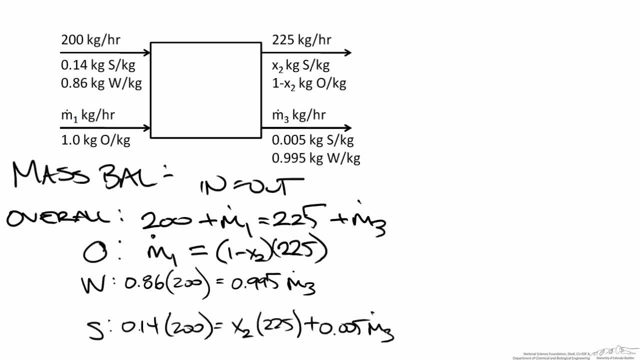 calculate what's been asked for. So, looking at the water balance, we can quickly calculate m3 and we can use the value of x2 times the total flow rate in the extract, which is m1.. So we have a value of m3 times the total flow rate in the extract, which is m1.. In doing the calculation, I 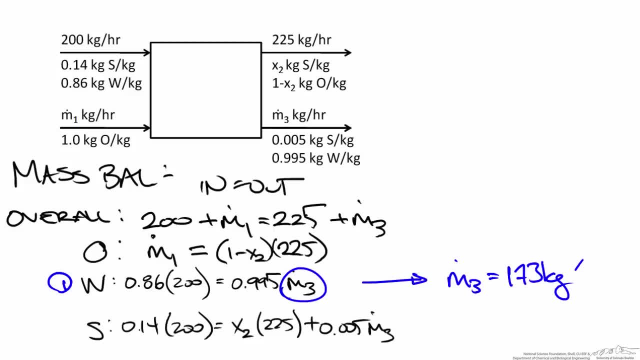 find a value of m3 is equal to 173 kilograms per hour. With the value of m3, we can then plug that into the overall balance and solve for m1, which is the first thing that we were asked for: Rearranging the overall balance to solve for m1, I get a value of 198 kilograms of organic solvent. 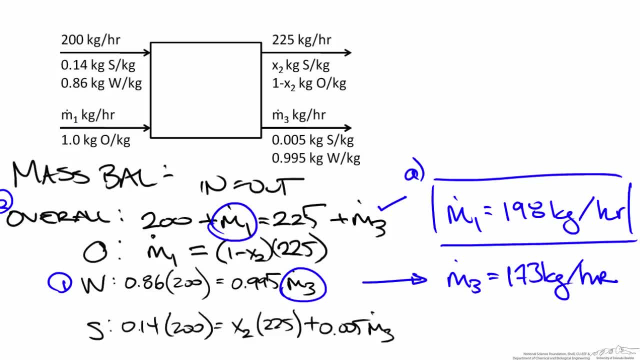 per hour. The second thing that we were asked to calculate was the recovery of the solute in the extract. so we need to calculate x2.. Here we have a value of x2 times the total flow rate. in Here we have a choice. we could use either O or S. Doesn't really matter which balance we use. 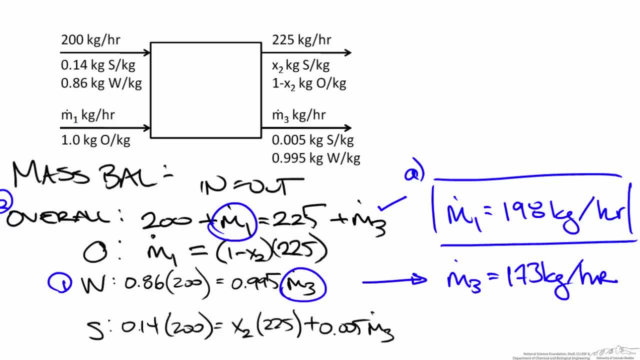 we should arrive at the same answer if we set the balances up correctly. So, as a matter of convenience, I will use the organic solvent balance. We just found. m1 was equal to 198 kilograms per hour, so the only unknown in this balance is x2.. Solving for x2 in this balance: